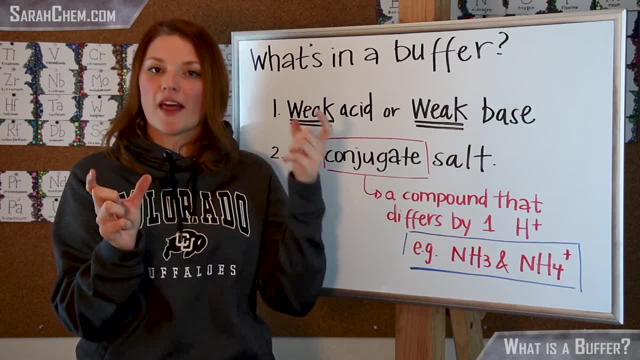 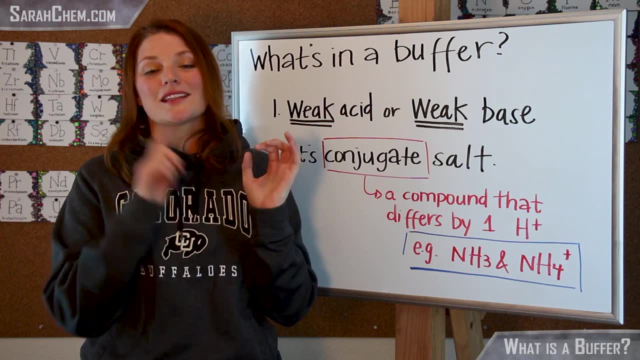 salt that you put in the solution that contains the conjugate of that weak acid or weak base. So just to make sure everyone's on the same page when we say conjugate, a conjugate is a compound that differs by one proton. So, for example, if we take a look at this, we 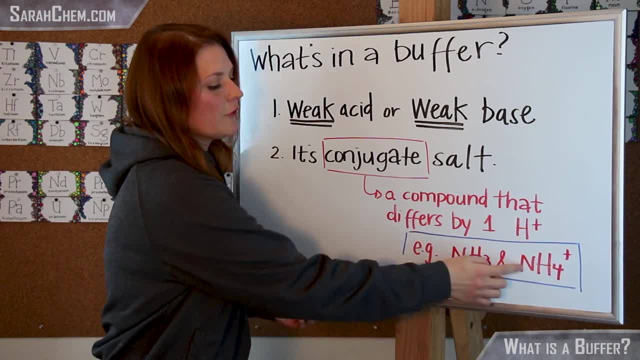 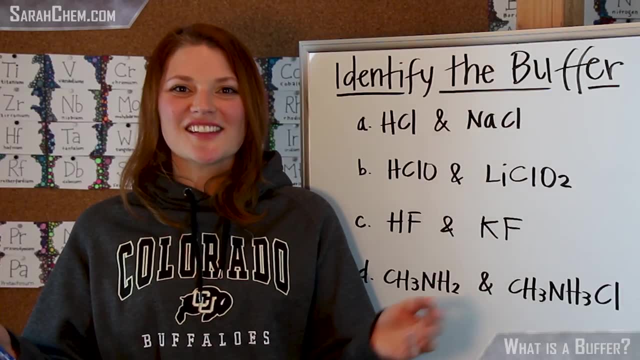 have ammonia and ammonium, And if you look at them, you can see that their formulas differ by one H plus, And because of that these two would be a conjugate pair. Okay, so now let's take a look at an example where we can actually utilize that information. 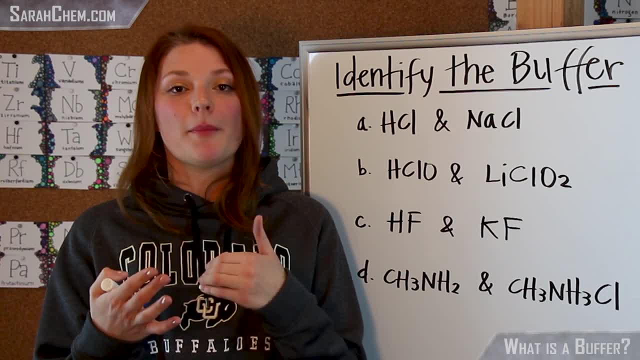 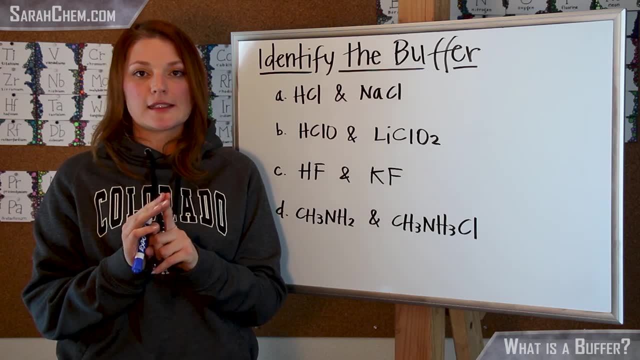 of what's in a buffer to identify whether a combination of compounds is a buffer. So remember, the two things we're looking for is one: is everything in there weak, no strong substances? And then, secondly, do we have a conjugate pair in solution? So let's use those two criteria to run. 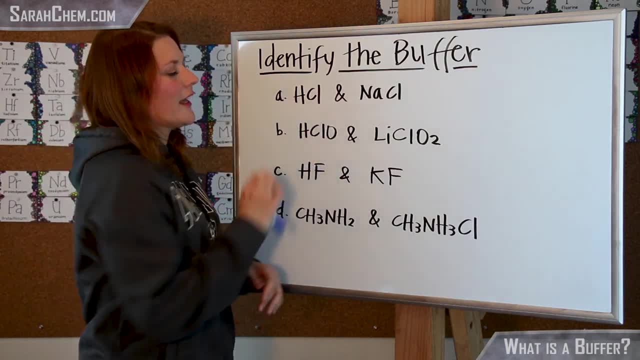 through this list. So if we take a look at A, the first thing I look at is HCl. So I recognize that HCl is a strong acid. Generally in your courses you're going to have either 6 to 8 or more HCl. 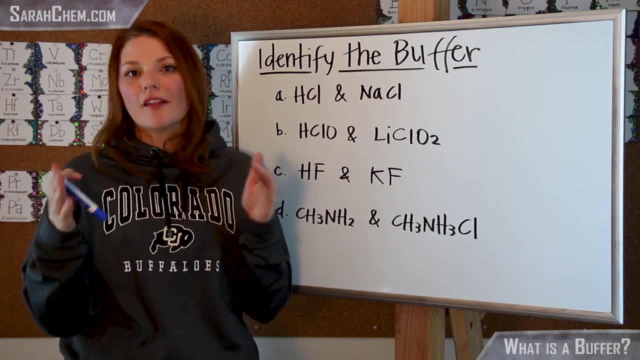 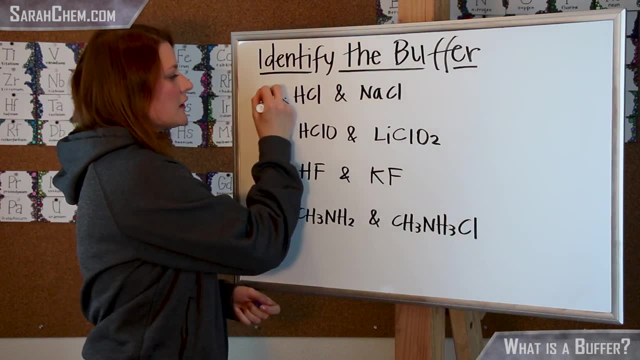 to eight strong acids that your teachers ask you to memorize, and if it's not on that list, then it's not a strong acid and you can assume it's weak. HCl is a strong acid, so automatically you can disqualify this without having to look. 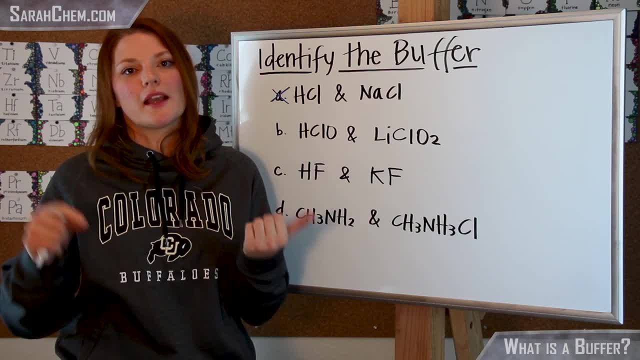 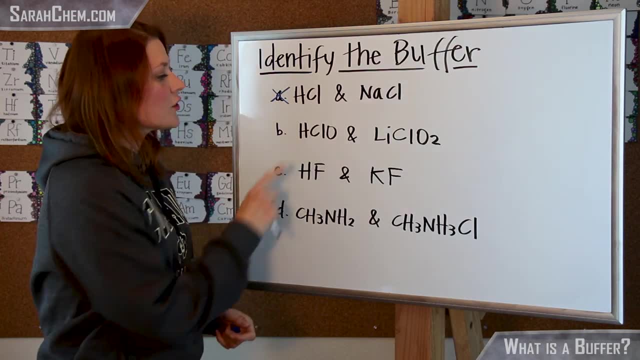 any further at whether you have a conjugate pair, because I know I cannot make a buffer with a strong acid. So then we move on Here. I look at HClO. So this here is a weak acid. so that means first criteria is met. So now I'm going to take 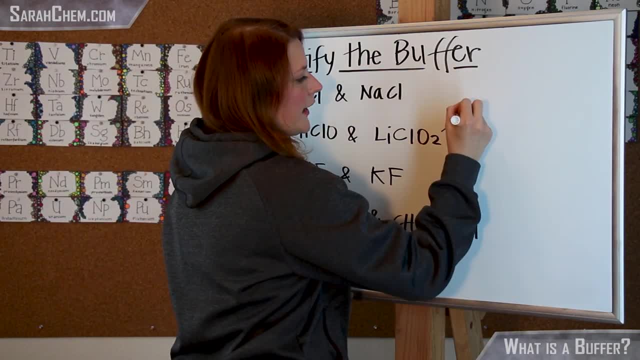 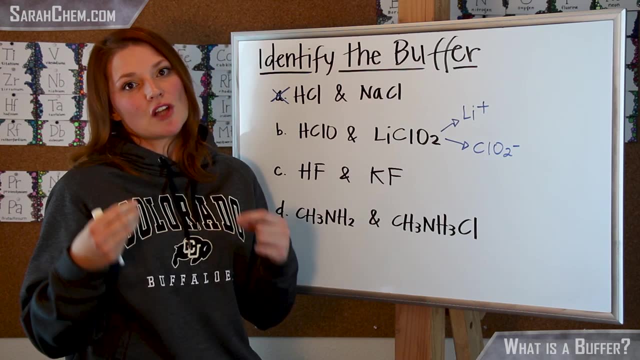 a look at this. Remember that this is a salt, so this is going to break up into Li plus and ClO2 minus. You might want to look at your polyatomic ions that you need to memorize in order to figure out how you'd know how to split this up. So 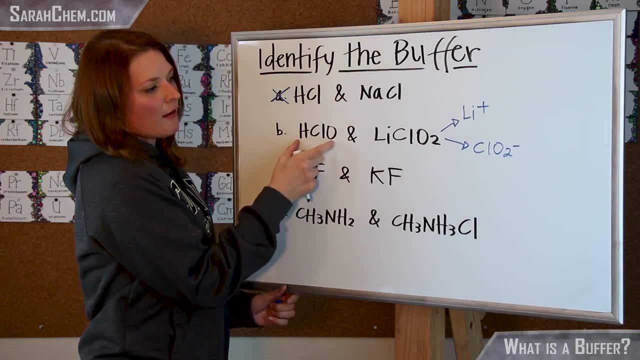 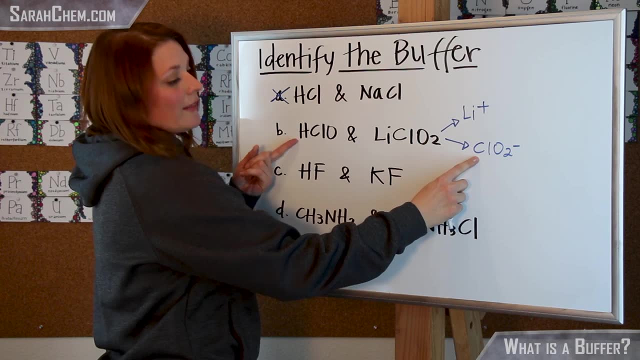 now, if I take a look at this one, I check to see is that the conjugate of this. So remember, conjugate means they differ by one hydrogen and one hydrogen alone. So this one has one less hydrogen than this one does, but this has two O's and this: 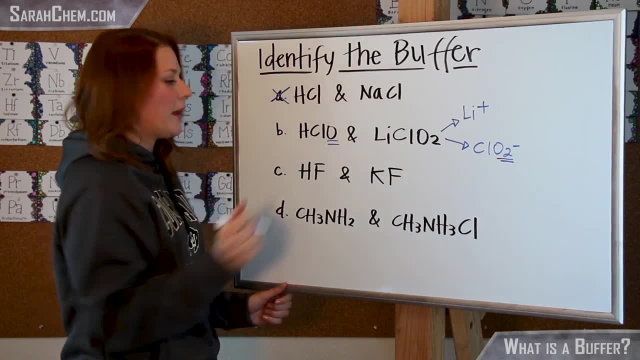 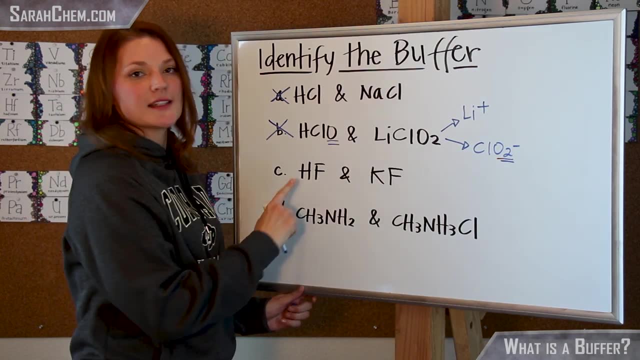 is a weak acid, So I know I'm going to have to go through this in a little bit- only has one. So this and this are not a conjugate pair, So this one also would not be a buffer. I take a look at this First criteria: Do I have a weak acid? Yes, I have a weak acid.